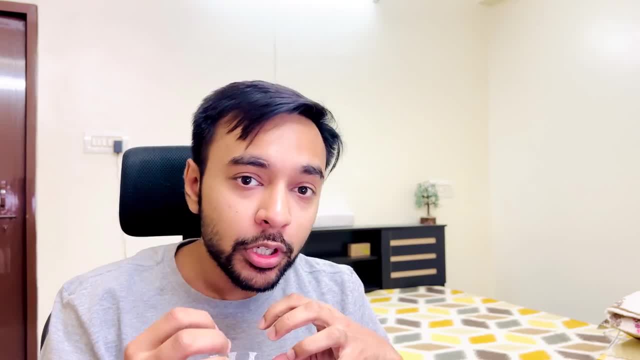 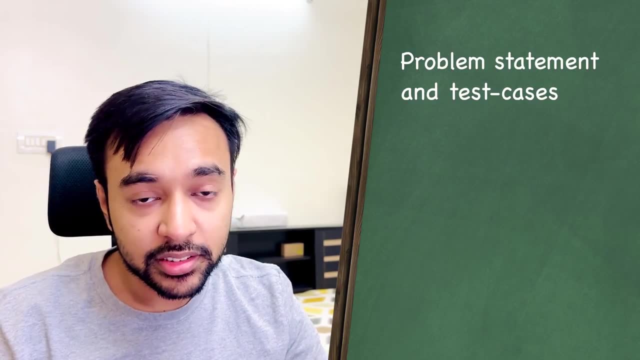 and how you can go step by step from ground up. So that is what we are going to do. Hello friends, welcome back to my channel. First I will explain you the problem statement and we will look at some sample test cases. Going forward, we will see why a brute force solution is not optimum and why a 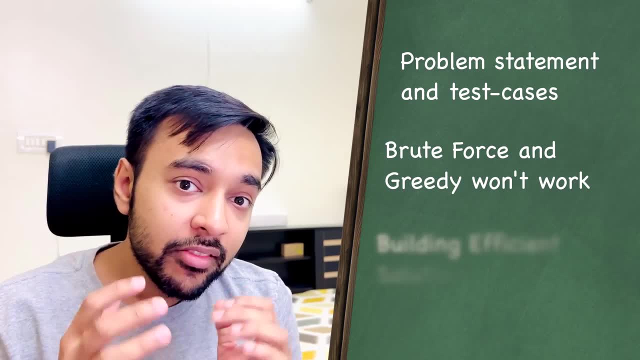 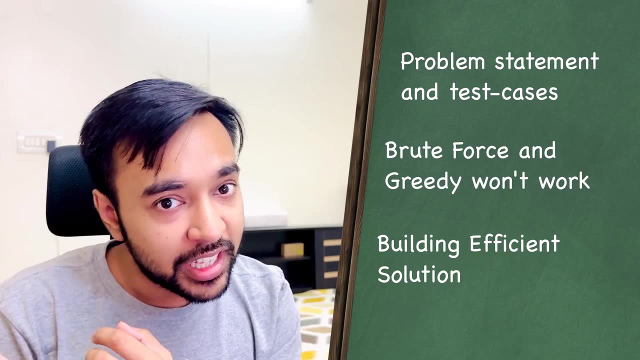 greedy approach will give you a wrong answer. Going forward, we will see how you can start from the ground zero and build up a dynamic solution, And after that, as usual, we will also do a dry run of the code so that you can understand how. 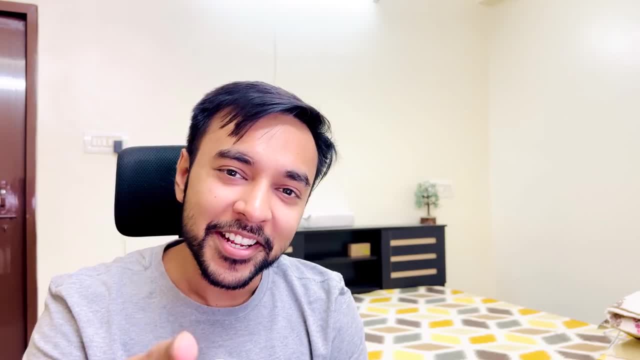 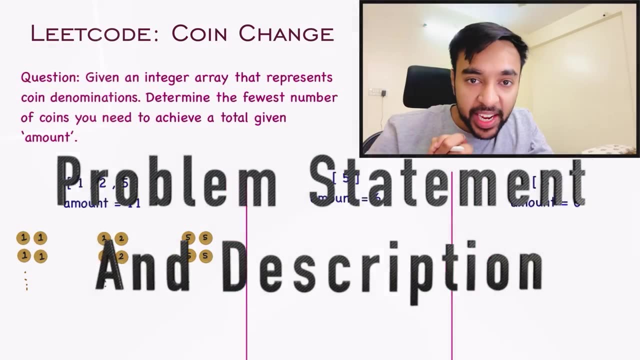 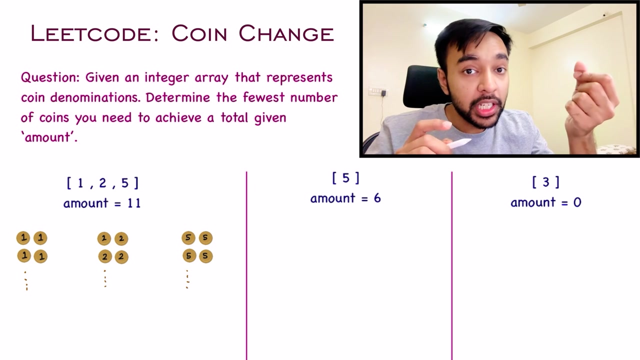 all of this actually works in action. Without further ado, let us get started. Let us quickly make sure that you understand the problem statement accurately. first, In this problem you are given an integer array that represents certain coin denominations. What does that mean? So a coin denomination of one means that you have some coins that have the. 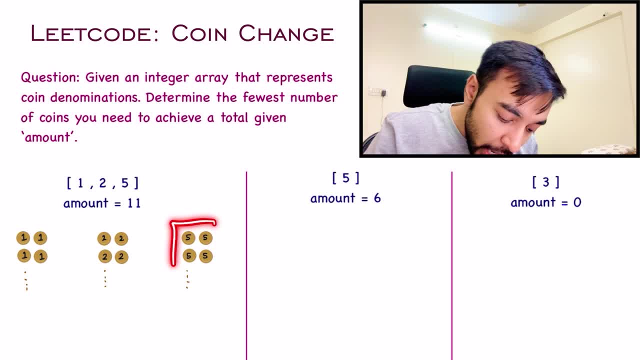 value one. A coin denomination of five will mean that you have some coins that have the value one. You have some coins that have the value five, correct? Now, given this array, you have to determine the fewest number of coins that you need to achieve a total given amount. So, for a test case, 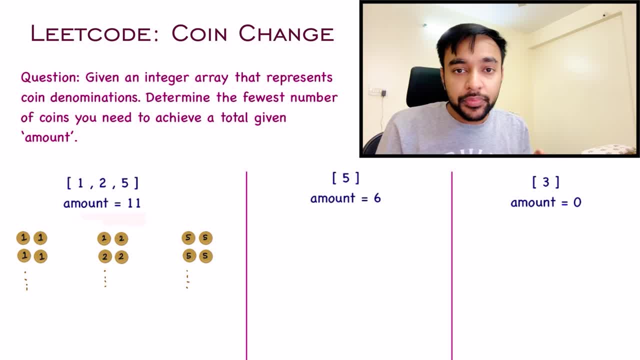 number one. I have to reach an amount of 11, right Now. now I ask you, how can you reach the amount 11?? If you choose only coins with the value one, you would need 11 of such coins. right, If I say: 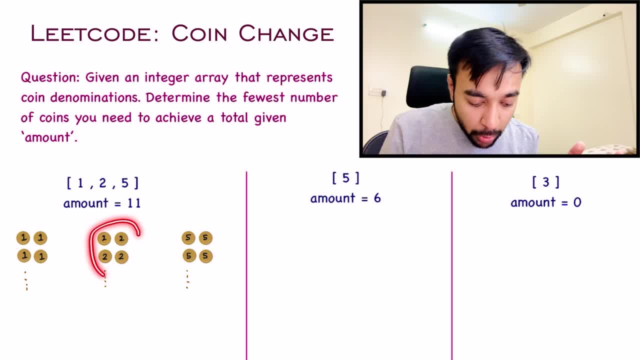 you that, okay, you can choose both one and two. then you will choose some coins of the value two and some coin of value one, right? So in this problem, if you have three such denominations- one, two and five- and you can assume that you have infinite number of coins. So what is the? 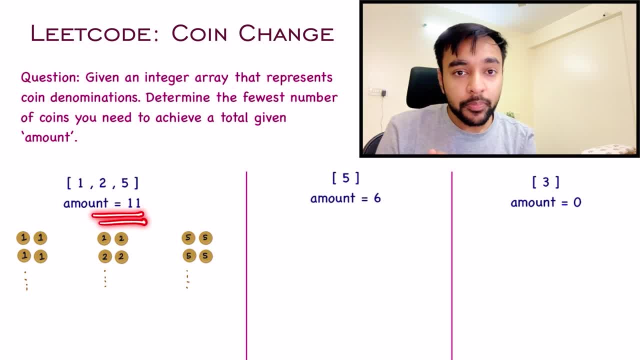 fewest number of coins that you need to achieve this value- 11?. So for this particular test case, you can achieve this value when you take up two coins of value five and you take up one coin of value one right. If you add them up, you get 11, right. So how many coins did you need? 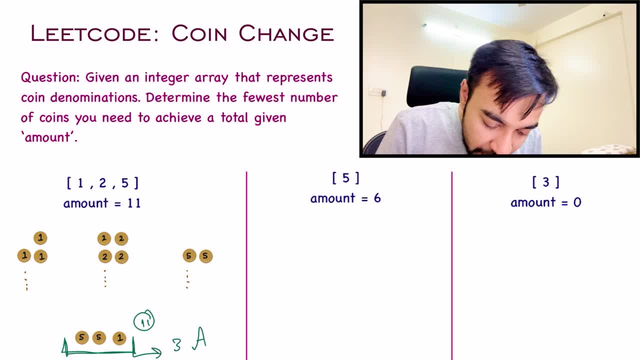 You needed a total of three coins, right? So three will be your answer. Similarly, let us look at our test case number two. In a test case number two, you only have the denomination five available, correct? And you have to make a total amount of 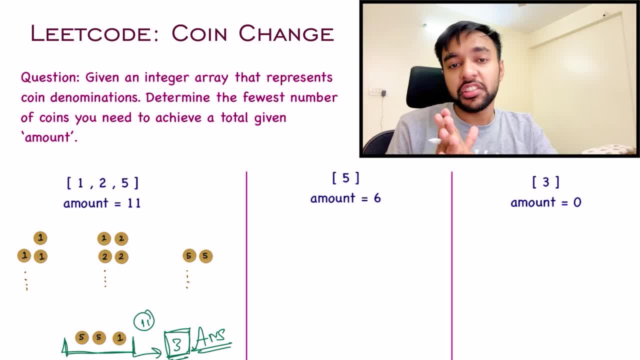 six. So if you notice, if you only have the denomination five, so how many amounts you can make, You can either make a five, or you can make 10, or you can make 15, right, You can never make amount that is six. So in such a case, when you cannot make that amount, 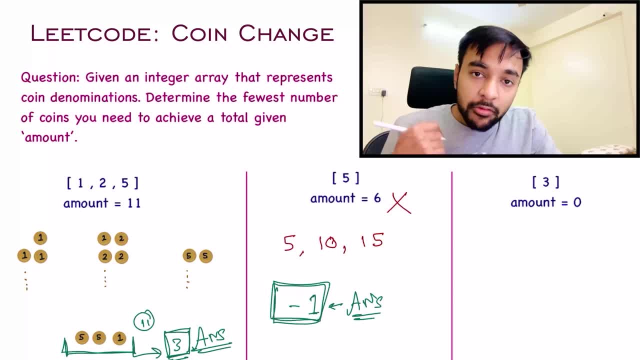 you have to return minus one as your answer. We also have one more special case. Suppose I have denominations of amount three and the total amount that I have to make is zero, So that case is also valid, And then you will not pick any coin. When you're not picking any coin, your default amount, 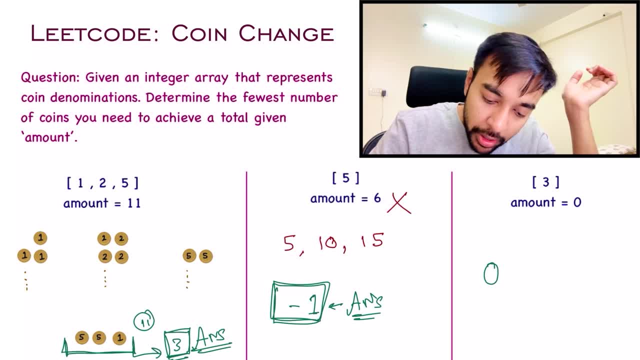 will be zero, right? So in this type of scenario, zero will be your answer. So now, if you feel that you have understood the problem statement even better, first feel free to try the problem on your own, Otherwise let us type in the answer. So, in this type of scenario, zero will be your answer. 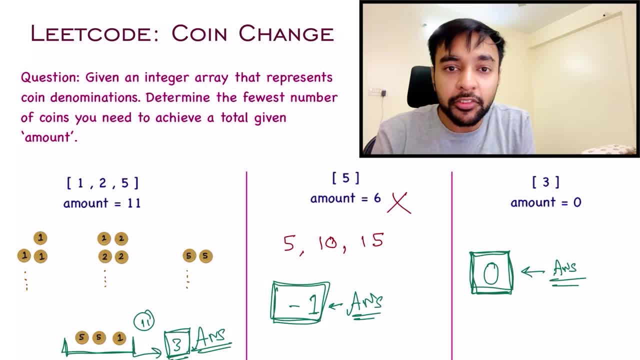 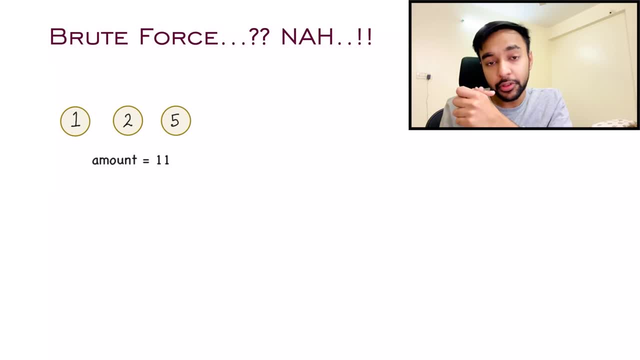 So let's dive into the solution and see how you can use the minimum number of coins to arrive at your answer. To start understanding things, let us take up the sample test case that we had available in the previous scenario, correct: You are given three denominations- one, two and five- and you: 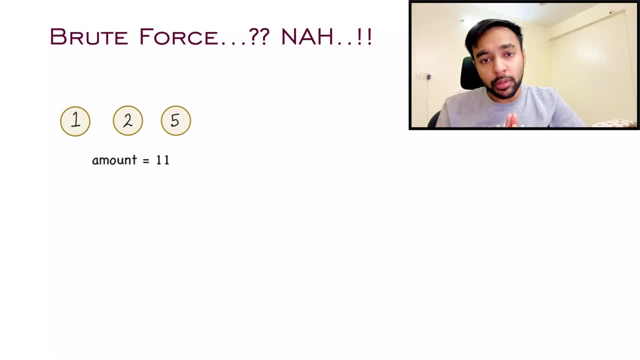 have to reach the amount 11.. So the brute force way to approach this problem will be that you will try all the possible combinations of all these three coins. You can start with coin two and then try different combinations of one and five. You can start with coin five and then try different. 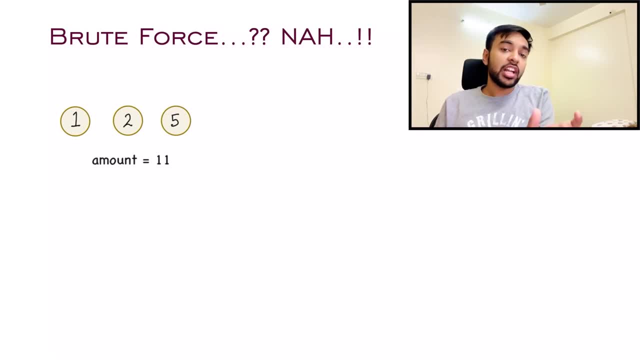 combinations of one and five. Now, if you see the computation of whole number of coins and try the algebra of half, If you see that with this combination of coins, if you need a minimum number of coins, you will see there. okay, with this combination I need the minimum number of coins. 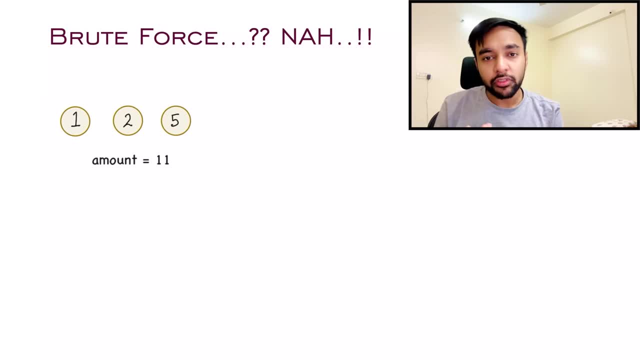 and that will be your answer right. Sure, that will give you a correct answer. But even for such small test case, it will end up taking a lot of time And you will have unnecessary number of combinations. you will waste so much time. So you are gonna think that, okay, I need to now optimize. 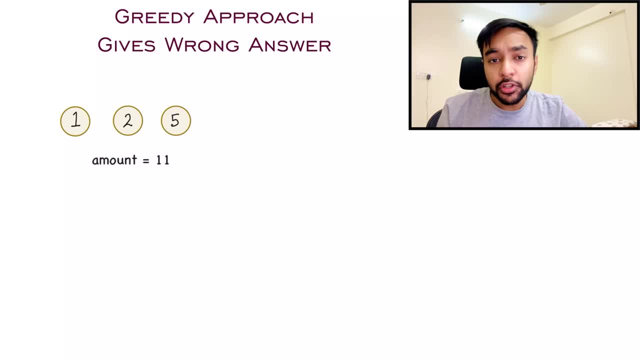 the solution And when you have to optimize, one approach that will come to your mind is: okay, how about a greedy approach? the link in the description below to one of my examples- so basically how the greedy approach will work- is: you have to achieve the minimum number of coins right and with these denominations. 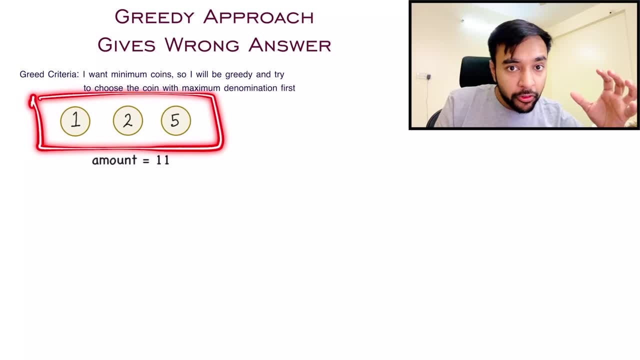 so a greedy approach will be that okay for minimum number of coins. what if i start with the maximum denomination? because a maximum value will keep on reducing this value. right, so what i can say is: okay, i take up one coin that is of denomination five and then my remaining. 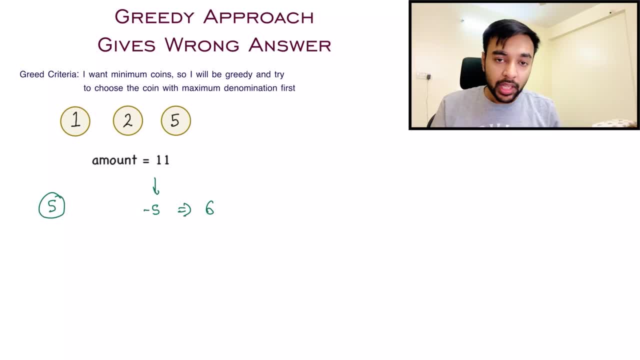 amount is equal to six, correct? so once again, you will see that, okay, if six is remaining, what all choices do i have, i can once again choose five, right? so what i'm gonna do is i will pick five again, and then how much amount am i remaining with? i'm remaining with one right. so now you. 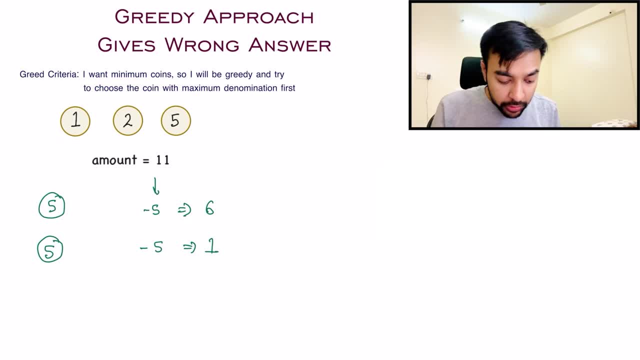 have three more choices and your remaining amount is only one. what you will see is: okay, i have one available and i will choose this coin. i choose this coin and then my remaining amount is zero. so how many coins did you use? you used a total of three coins, and voila this. 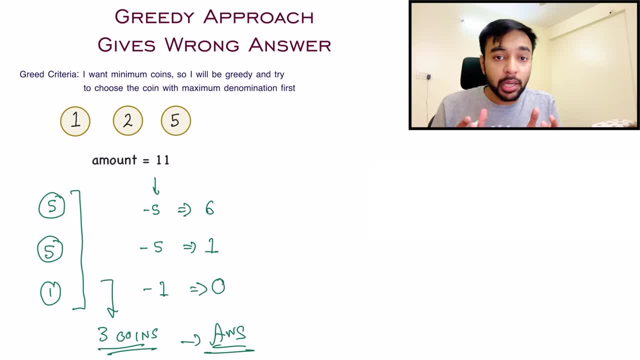 is the answer right and you may feel that, okay, a greedy approach works. but there could be some scenarios possible where a greedy approach can give you a wrong answer. for example, let us take up this sample test case. this time i have denominations one, five, six and nine and once. 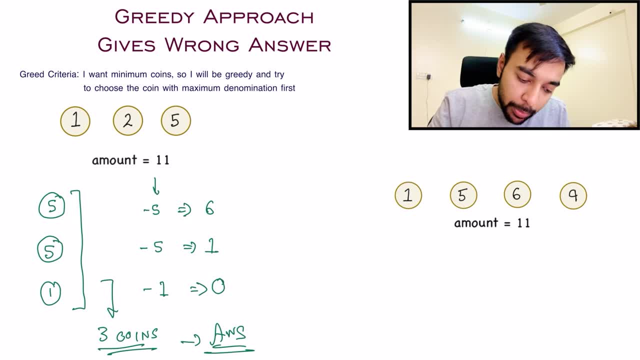 again, i have to reach the amount eleven. so, following the greedy approach, what i'm gonna do is i'm gonna choose the amount of coins that i have available- nine, right. so i choose a point nine and my remaining amount is two. now, when my remaining amount is two, what coin can i choose? 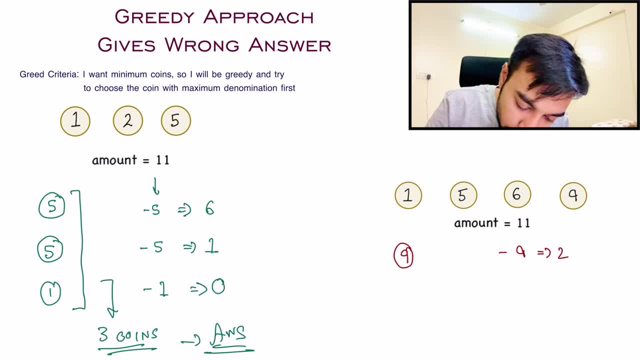 i can only choose coin number one, correct? so i choose the coin with the denomination one and i have a remaining amount of one again. once again, i will choose the coin with denomination one and i have a remaining amount of zero. so how many coins did i end up choosing? i took a total of three. 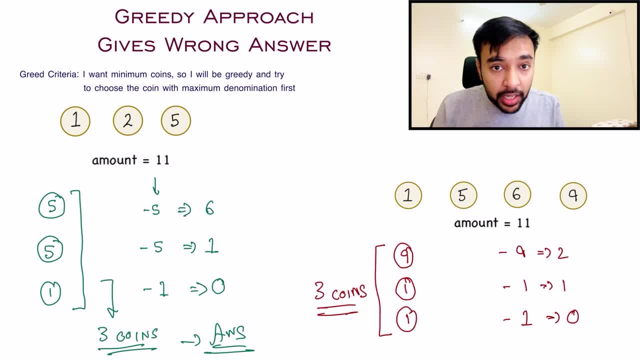 correct. it may feel that this is the correct answer, but if you notice closely, you can achieve this amount eleven if you choose only two coins, that is, one coin of the denomination five and one coin of denomination six. right, and in fact two is the correct answer. so you see why the greedy 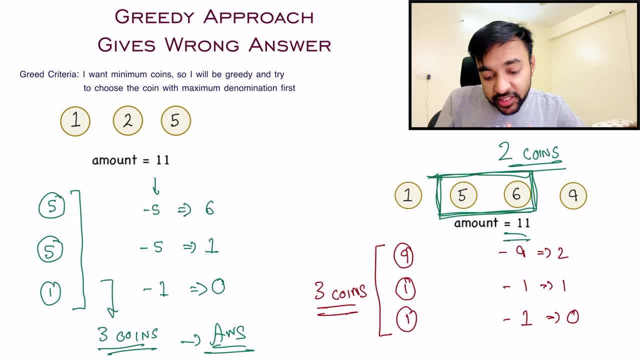 approach will not work for this problem. so that means you have to apply dynamic programming, because as the number of coins increase, you need to determine: okay, if i have some remaining value, what is the minimum amount of coins that i need to obtain, that you do not want to calculate everything again and again and that tells you that is a optimal. 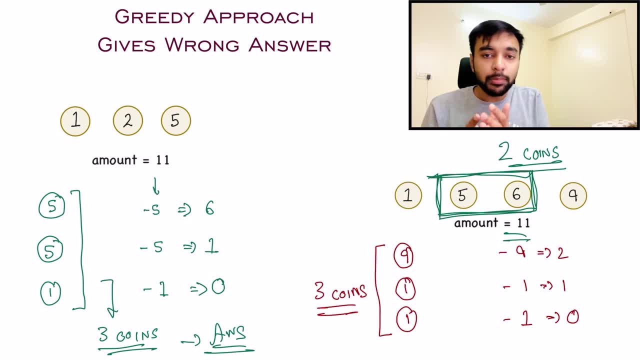 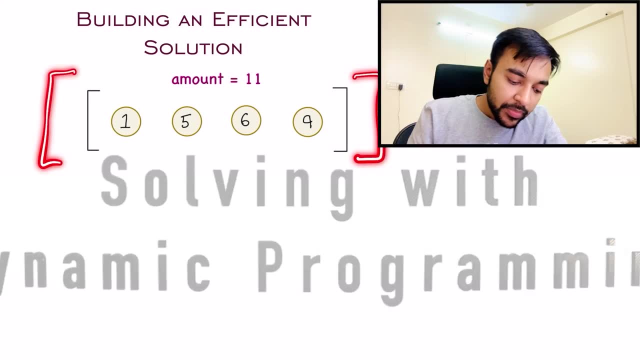 substructure property. it is a repeating pattern and it will be solved by dynamic programming. so what can we do about it? okay, so let us take up our sample test case once again. right, and this time i have four different denominations and i have to arrive at the. 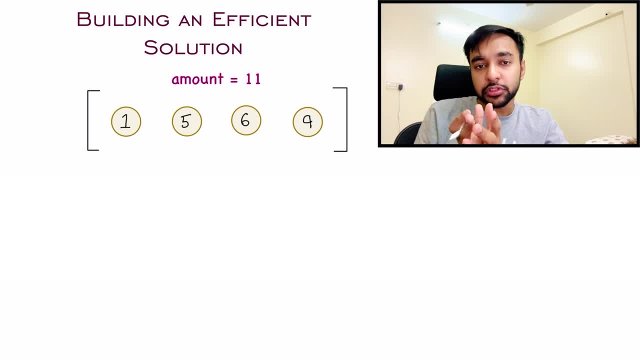 total amount eleven correct. when he was trying to solve the problem via brute force method. what was the problem that you were facing? the problem that you are facing is that? okay, if i pick the coin nine, my remaining amount will be two correct. so now to determine how many minimum. 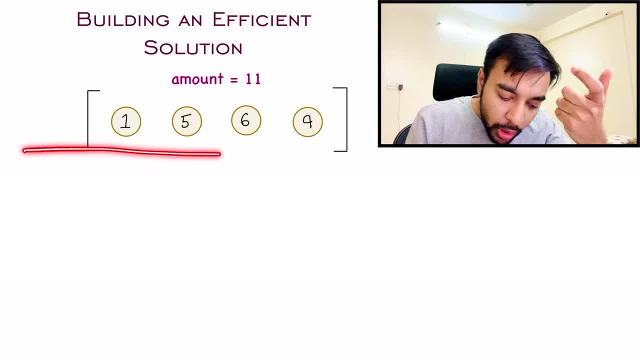 number of coins, you need to make the amount two. you once again have to iterate through all the possible choices, right? similarly, if you say that, okay, i will start with coin number six, correct? so what is your remaining amount? your remaining amount will be five, right? so once again, you have 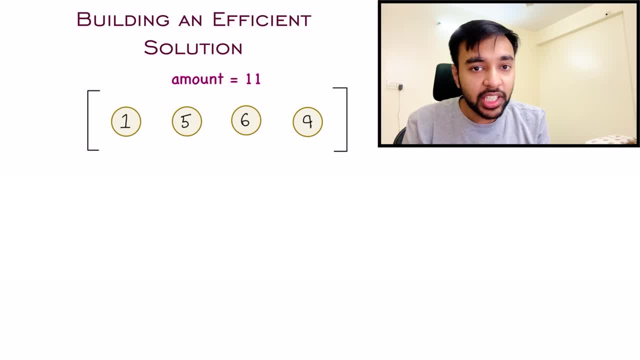 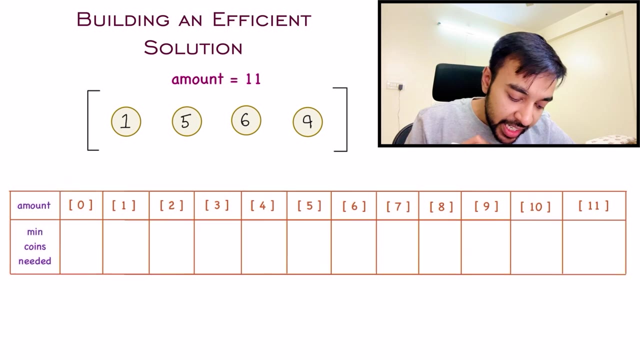 problem, just to see that. okay, what is the minimum amount of coins that i need to arrive at the remaining amount? five, correct. so this is what we will try to build our solution on, and this is the intuition and the idea behind this approach. so what i'm gonna do is i will create this array. 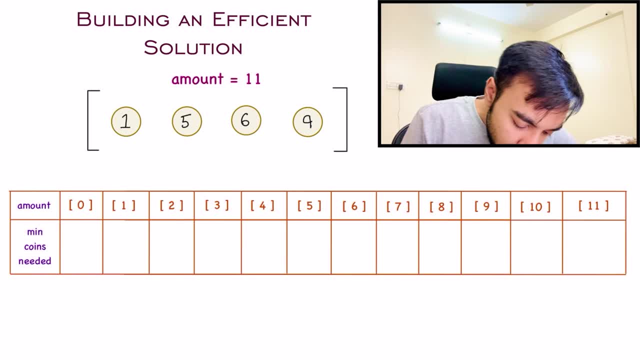 and in this array, what i will try to determine is how many minimum number of coins do i need to make the amount zero, to make the amount one, to make the amount two, then three, then all the way up to 11.. so, at every instance, this table will tell me that, okay to make the amount four. what is the 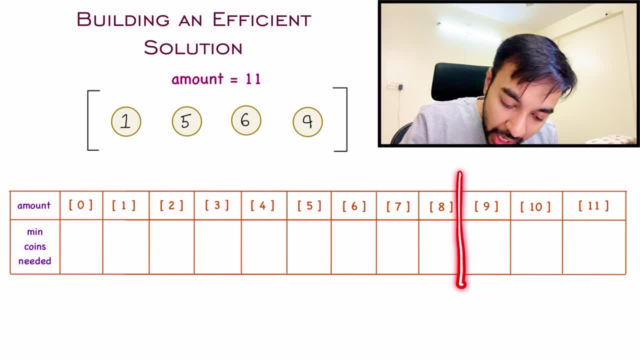 minimum number of coins that i need to make the amount nine. what is the minimum number of coins that i will need? so this is what this array will represent, but the real challenge is: how do you go about populating this array? i want to go real slow so that you can understand what is happening over. 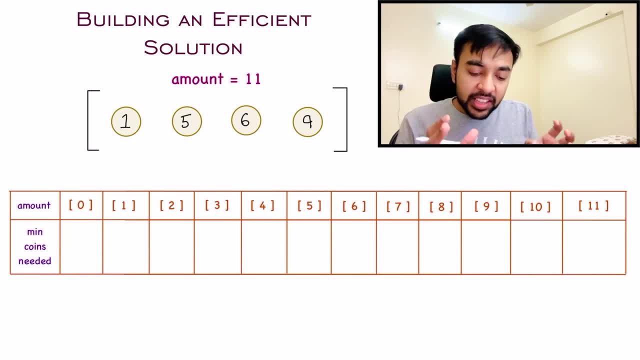 here, because there are a lot of problems for dynamic programming that are happening over here. so let's go ahead and start by making a zero amount. that will follow the same pattern. so always watch out for it and try to identify this pattern. so let us start off things. so, if you want, 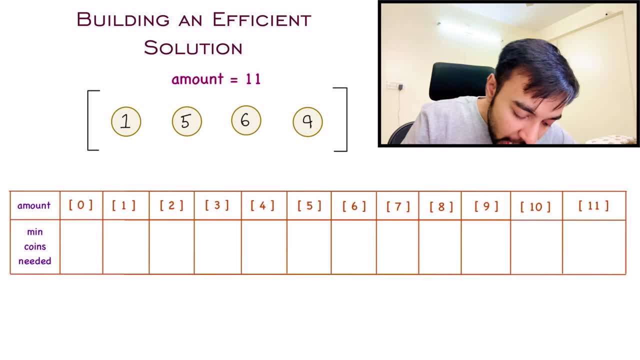 to make a zero amount. how many coins do you need? when you are making an amount zero, you do not need any coins at all, right? so i will leave this place blank because i do not need any coins. and then i have amount zero, correct. moving on to our next amount, this amount is one, so how many coins do you? 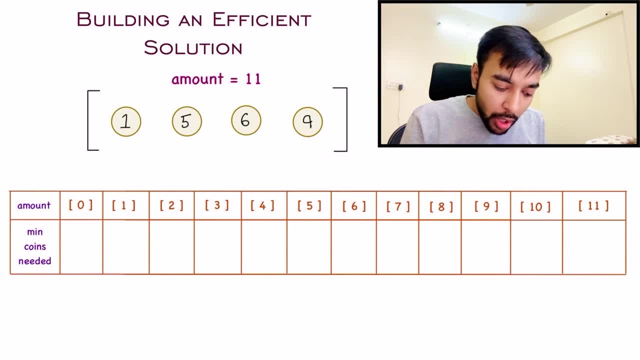 need. so you see that you have four coins: one, five, six and nine. all these three coins are greater than one, right, so you cannot pick them at all. you can only pick this minimum denomination coin right. and how many of them do you need? you only need one coin, correct? so this table is telling me that to 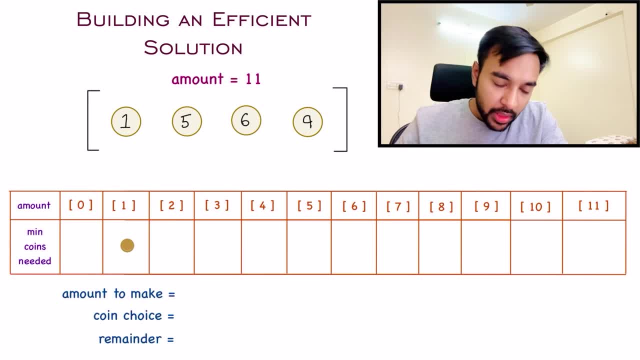 make the amount one. i only need one coin right now. move on to your next amount. what is the amount that you have to make? you have to make the amount two correct, and what coins you can choose. you cannot start with nine, you cannot start with six, you cannot start with five. 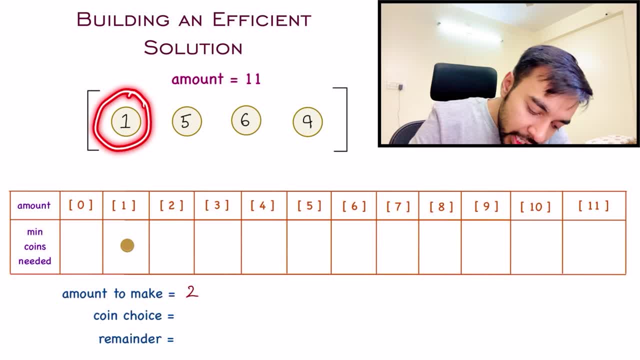 because all of them are greater than two right. you can once again only start with coin one right, so what i do is i start with my coin one, correct? so when i start with coin one, what is the remaining amount left? i still have to make one right, and now this is where 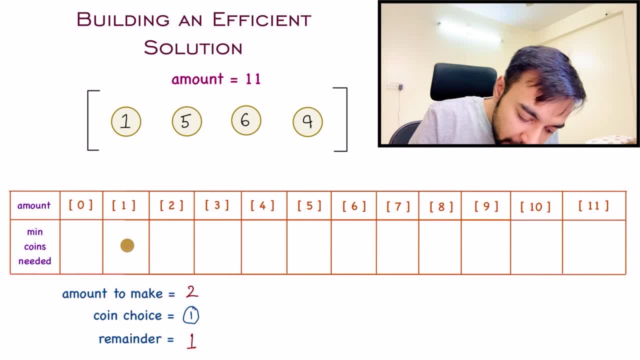 this table comes in handy. how many coins did you need when you had to make the amount one? you only needed one more coin, right? so we are gonna use this value over here. so how many coins did you use? one coin that you took and this one more coin from this table to make the amount one. 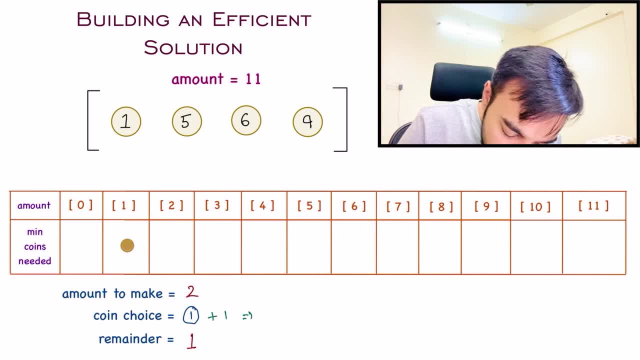 so that means that you will need a total of two coins to make the amount two right. just wait for a little while and follow along. things will become more and more clear in a while. now, what is the next amount that you want to make? you want to try and make the amount three correct. 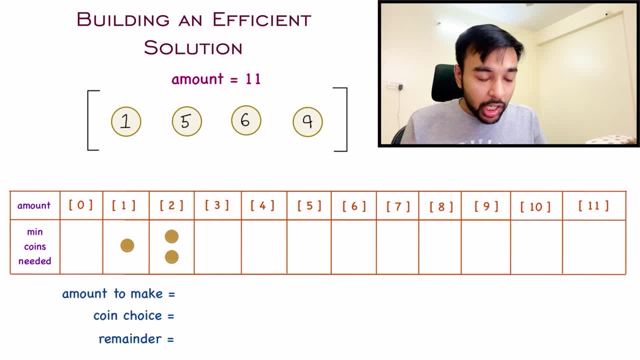 once again. nine, six and five are greater than three, so you cannot even pick those points once again. what happens is you have to make the amount three and the coin choice will be just one right, because you can start with the first coin. what is the remaining amount that you have to make? 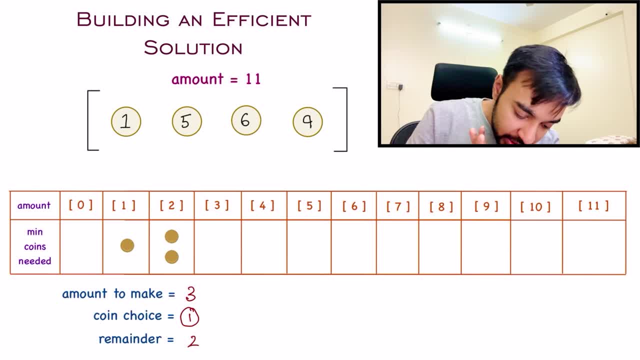 that will be three minus one, and that is two, correct? this is where, once again, your table comes in handy. check: how many coins do you need when you have to make the amount two? you needed a total of two coins, correct? so how many total points will you need? 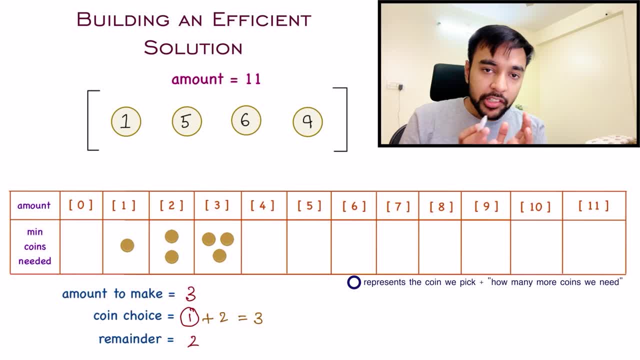 you will need one plus two, and that is equal to three coins. if you start looking at it, this is making sense right. to make amount one, you needed just one coin. to make an amount two, you needed a minimum of two coins. to make an amount three, you needed a minimum of three coins. 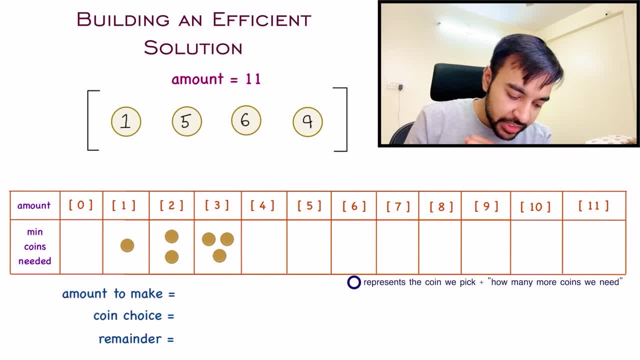 right, let us keep doing it and you will realize how beautiful this solution is. now move on to the next amount, and that is four. you have to make a total amount of four. once again, what coin can you choose? you cannot choose any of these three coins because they are greater than 4.. 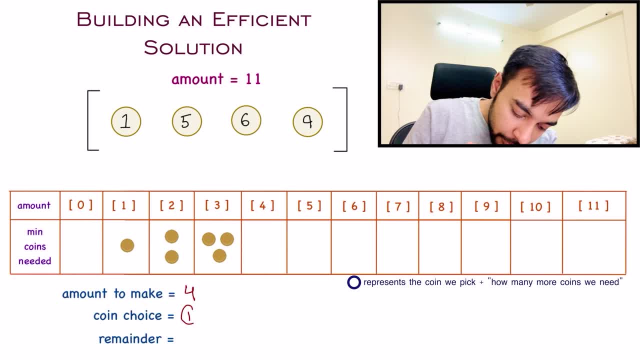 so there you go, you are left with just one right. so i take up this one coin, and what is the remaining amount that you have to make? i still have to make a remaining amount of three, and how many coins do you need to make this remaining amount? that is a total of three coins right? so i will add this: 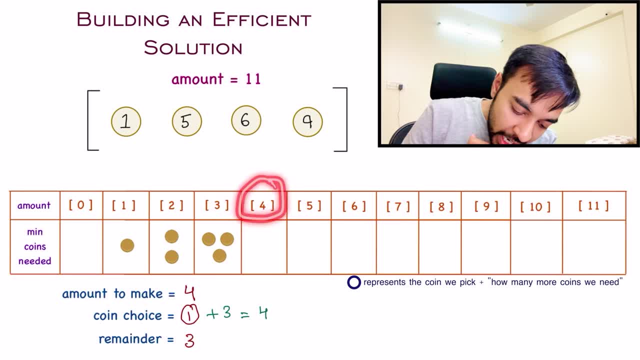 three over here and that gives me four. so to make amount of four, i need a total of four coins. if you have understood so far, trust me, half of the problem is already done. now. what is the next amount that you have to make? an amount of five, right? so this is where things will be very, very interesting, and watch closely. 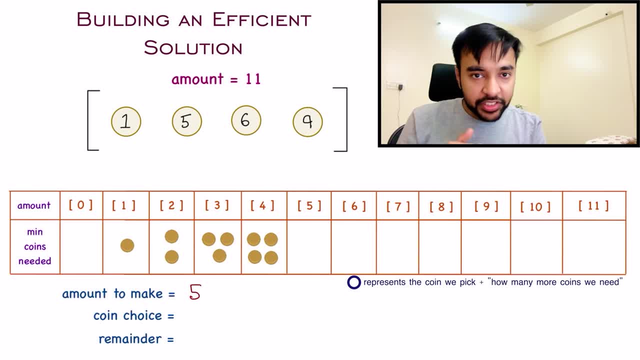 you have to make an amount of five, and what coins can you choose? you cannot choose nine, you cannot choose six, correct? but this time you have two coins to choose from. you can either choose coin five or you can choose coin one, correct. so what will happen is my coin choice will now be divided. 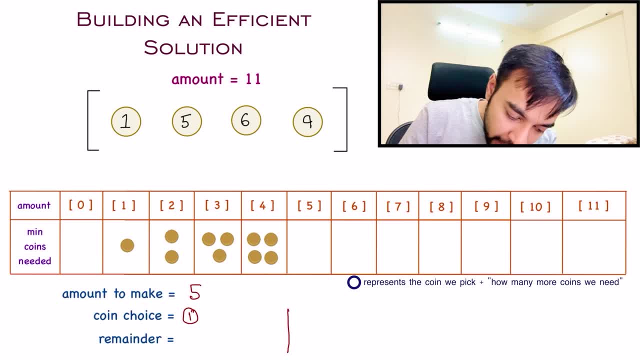 into two cases: one when i'm choosing coin one, and one when i'm choosing coin five. right, and now check what is the remaining amount in both of these cases. when i pick coin one, the remaining amount will be five minus one, and that is four. right to make this four remainder, how many more points? 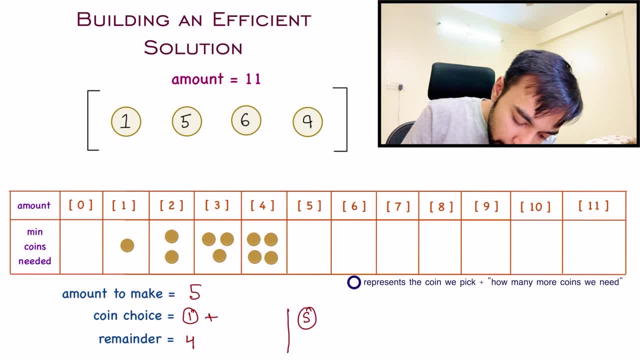 will i need? i will need four more points, right, so one plus four, and that will be five. so if my coin choice is one, then i will need five minimum points, right. but there is one more scenario: What if we chose 5 as the first coin? 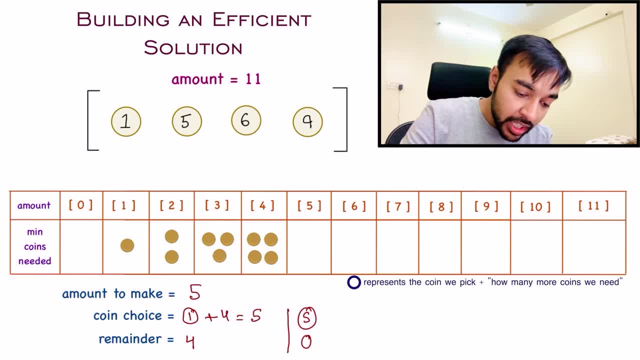 Then what is the remaining amount? Your remaining amount is 0, correct? That means you only chose 1 coin if you had to make a total of 5.. To fill this value now, you need to pick a minimum of both of these values. 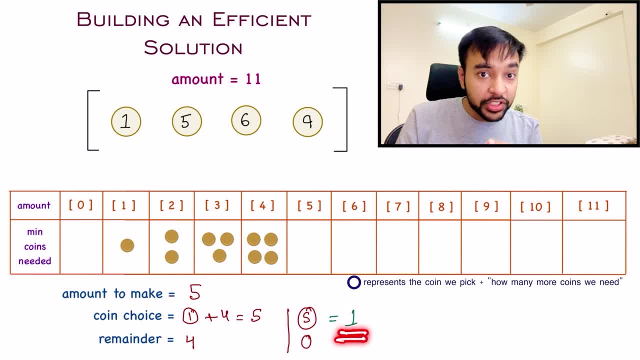 The minimum value is 1, right, Because you have to choose the fewest number of coins possible. So that means to make the amount 5, I only need 1 coin right Now. let us keep moving along, And this time we will try to make the amount 6.. 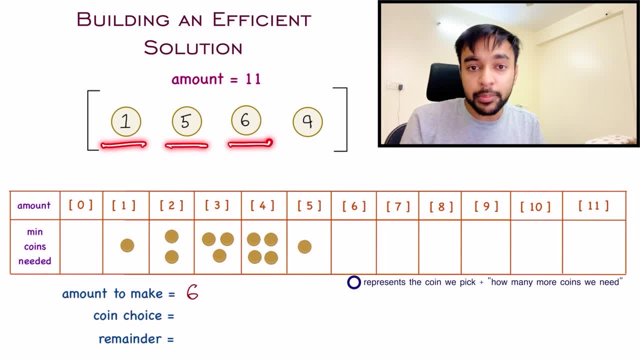 To make the amount 6,, you will see that I have 3 coin choices. this time I can start with any of them. So I have a coin choice of 1,, I have a coin choice of 5, and I have a coin choice of 6,, correct? 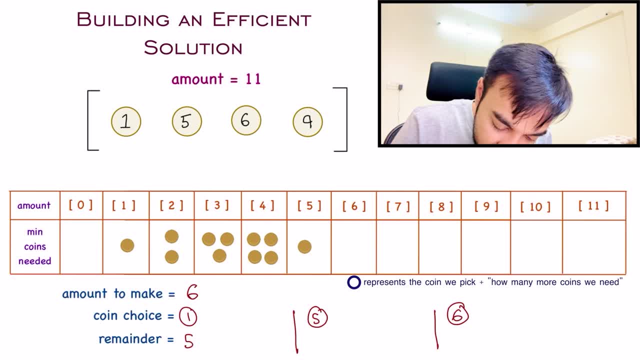 And what is the remainder amount? Remainder amount is 5 in this case, remainder amount is 1 in this case and remainder amount is 0 when you have to make a total amount of 6, correct? And how do you make these remainders? 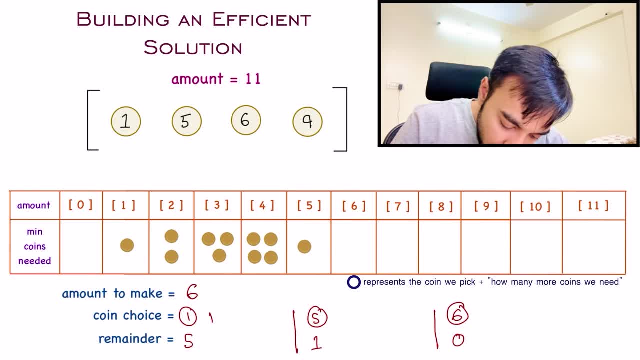 To make a remaining amount of 5, you will need 1 coin, so I am going to add 1 over here. To make a remainder amount of 1, once again, you will need 1 more coin, so I will add 1.. 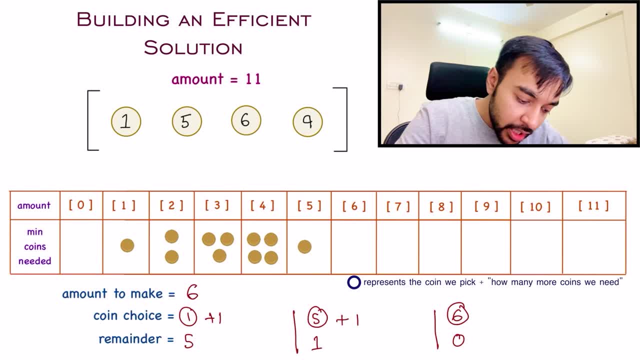 And to make a remainder amount of 0, you will need 0 more coins. So in this case you will only need 1 coin in total right. So out of all of these 3 values, what is the minimum number of coins that you need? 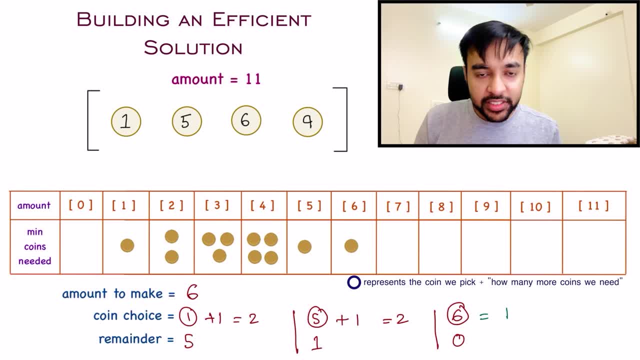 That will be 1 again, correct? So once again, try to visualize this array. If you wanted a total amount of 6, how many minimum number of coins that you need? You only need 1 coin That will be of denomination 6.. 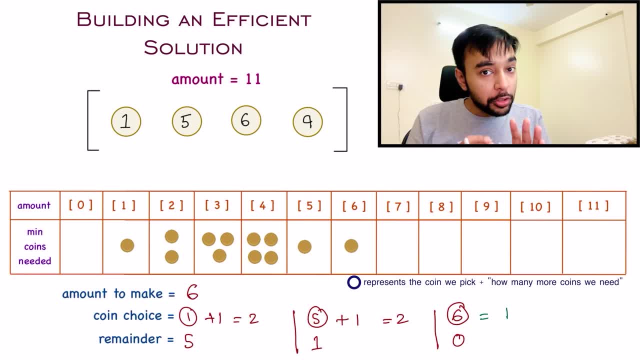 If you wanted to make a total amount of 4, how many coins will you need? You will need at least 4 coins. Similarly, for 5, you will need just 1 coin, and that is the denomination of 5.. 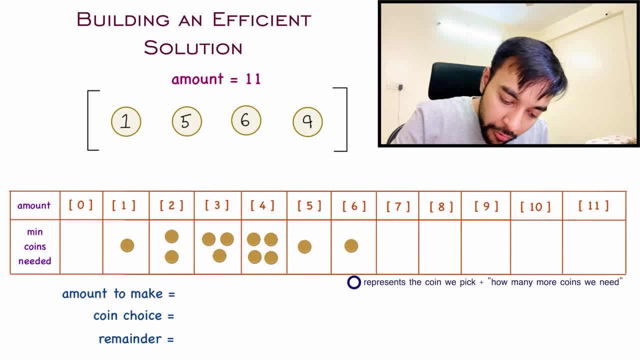 I will just keep moving along and do this example for value 7 onwards. This time I have to make the value 7, right And I have 3 choices available: 1,, 5, and 6.. I still cannot pick up 9 because it is greater than 7.. 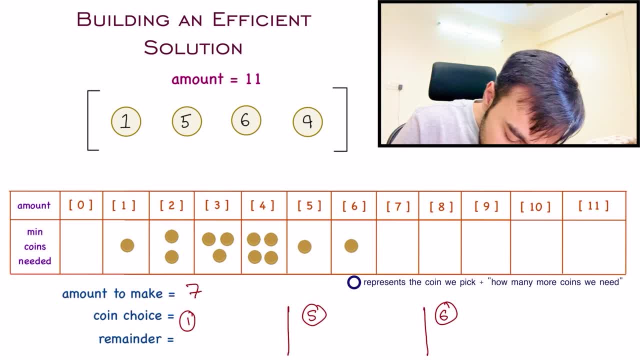 So I have 3 choices. And in all these choices, what is the remaining amount? 7 minus 7.. 7 minus 1, that is, 6.. 7 minus 5 will be 2.. And 7 minus 6 will be 1.. 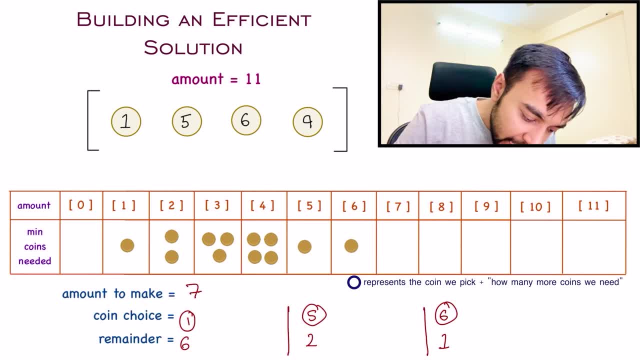 To make these remaining amounts. how many more coins do I need For 6, I will just need 1 more coin For 2,. I will need 2 more coins For 1,. I will need just 1 more coin. 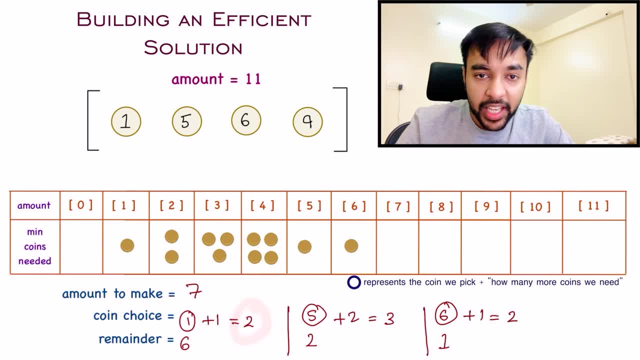 Out of these 3, what is the minimum value? The minimum value is 2 again. So to make a total of 7, you will need a minimum of 2 coins. Moving on to our next example, when I want to make a total of 8.. 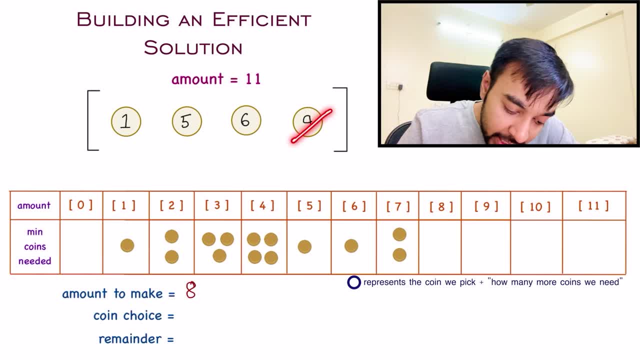 I will once again have 3 choices: 1,, 5, and 6.. See that I still cannot pick up 9.. So I am either choosing 1,, or I am choosing 5,, or I am choosing 6.. 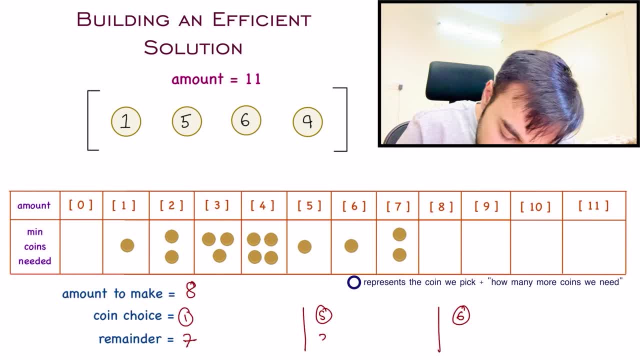 Then the remainder amounts will be 8 minus 1, 7.. 8 minus 5, 3. And 8 minus 6, 2.. So the total coins needed to make a remainder amount of 7 will be 2.. 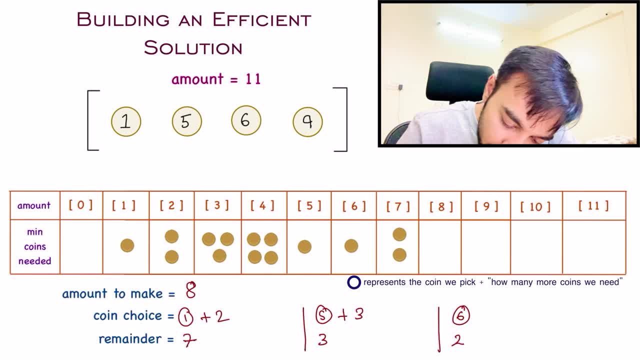 To make a remainder amount of 3 will be plus 3.. And to make a remainder amount of 2 will be plus 2.. Out of all of these, what is the minimum value? That is, 3.. So to make a total amount of 8,. 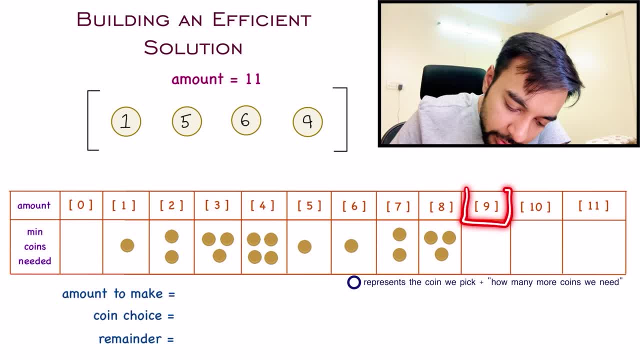 I will need 3 coins, Working out the next case, when I have to make a total amount of 9.. This time I have to make an amount of 9.. And what are the coin choices available? This time I can choose any of the 4 coins to begin with. 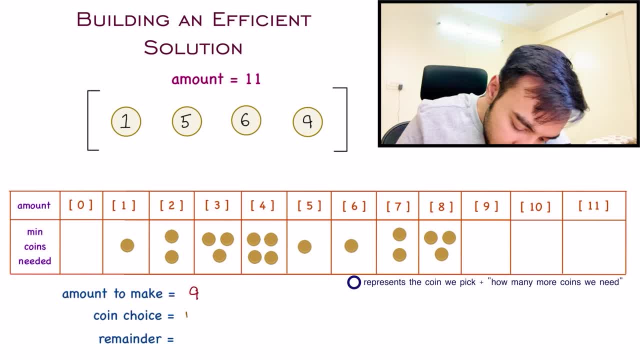 Right, And this case is also interesting. So I can either choose 1, or I can choose 5,, or I can choose 6, or I can choose 9.. Correct, And in each of these cases, what is the remainder amount? 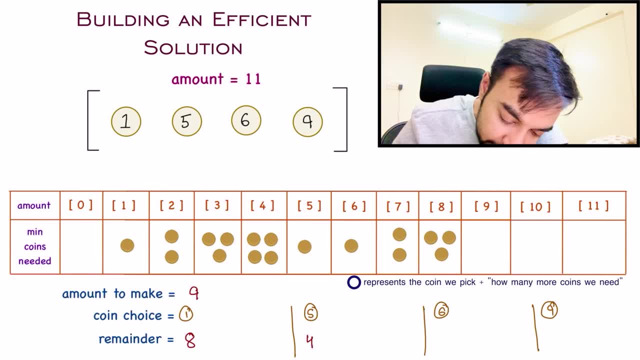 I have 8 remaining: in the first case, 9 minus 5, 4. in the second case, 9 minus 5, 4 in the second case, 9 minus 6, 3 in the third case And 9 minus 9, 0 in the last case. 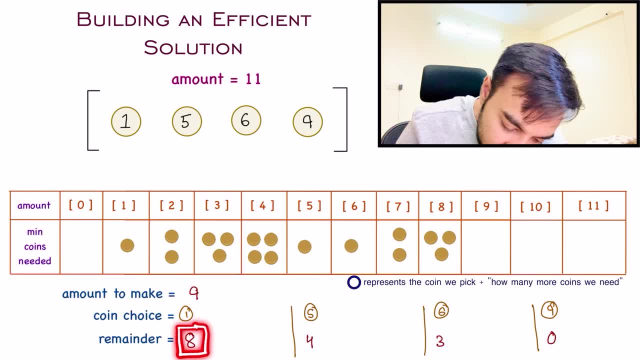 Next you have to determine: okay, how many coins do you need to make the remainder amount of 8? And that will be 3 more coins, So that turns out to be 4.. To make a remainder of 4,, you need 4 more coins. 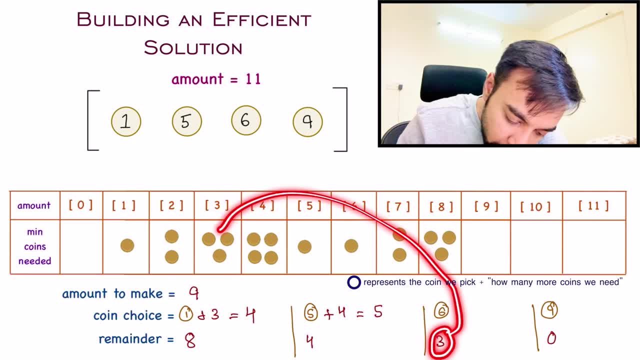 So that will be 5.. To make a remainder of 3, you will need 3 more coins. And then to make a remainder of 0, you do not need any more coins. So in the last case you only need 1 coin. 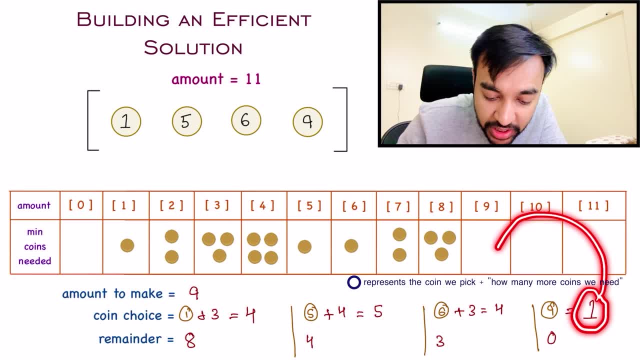 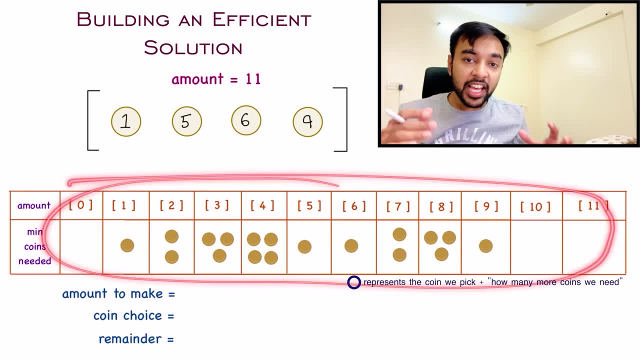 So once again, you can see that to make an amount of 9, you just need 1 coin. So you can see how we are reusing all of our solution right. This array is doing memoization And we are storing the result: how many minimum number of coins that we need to make each of these amounts correct. 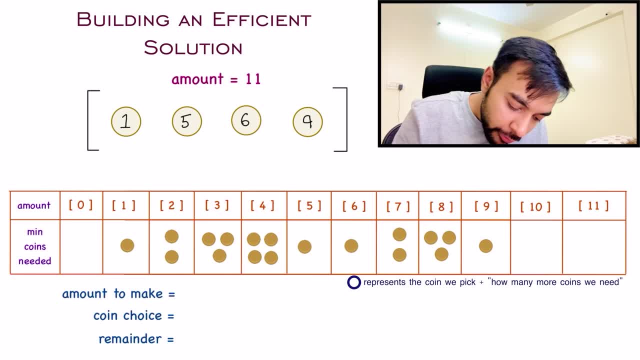 Let me just finish up this problem. To make the next amount 10,. what do I have? I have to make the amount 10.. And once again, I can choose either of these points to start with. For remainder of 9,, how many coins more do you need? 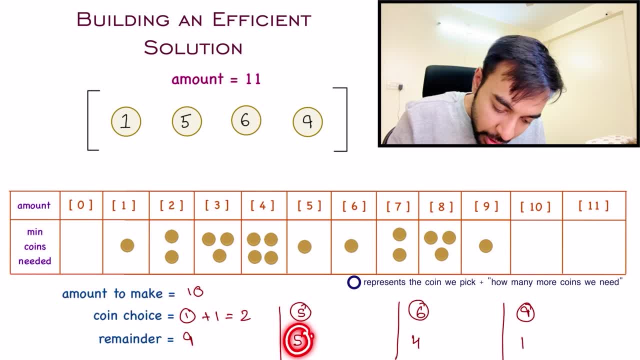 You need 1 more coin, So that would be a total of 2 coins. For a remainder of 5, you just need 1 more coin, So that will be once again 2.. For a remainder of 4, you need 4 more coins. 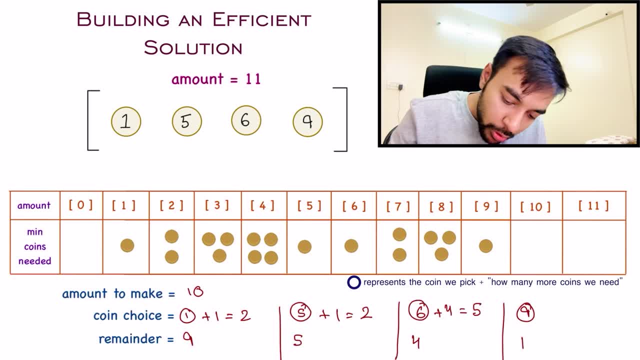 So that will be 5.. For a remainder of 1, you need just 1 more coin, So that would be 1.. And that gives you 2 again. Out of all of these 4 values, the minimum is 2.. 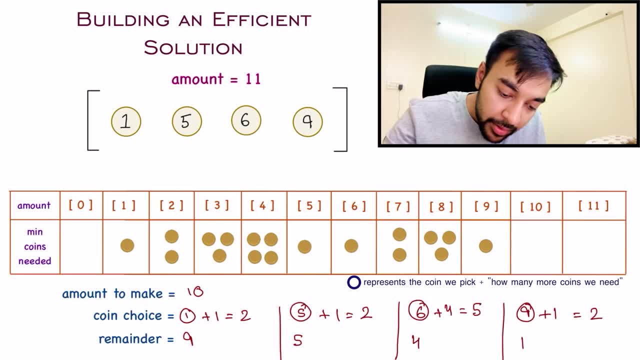 So that means I need a minimum of 2 coins to make the amount 10.. So you see how we stored all of our results And ultimately, let us try to see how many minimum number of coins do you need to arrive at the amount 11.. 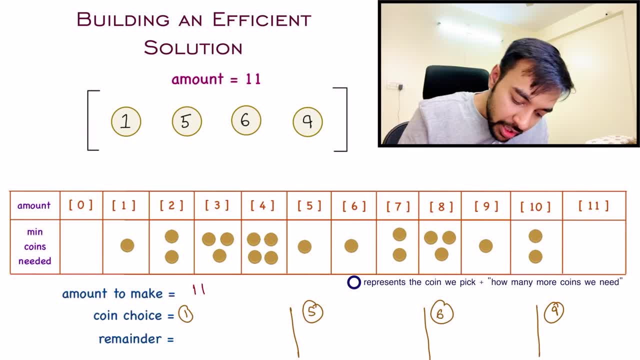 And you can choose any of the 4 coins to begin with. And what is the remainder amount? To make this remainder amount of 10,, you need a total of 2 more coins. To make a total of 6,, you need just 1 more coin. 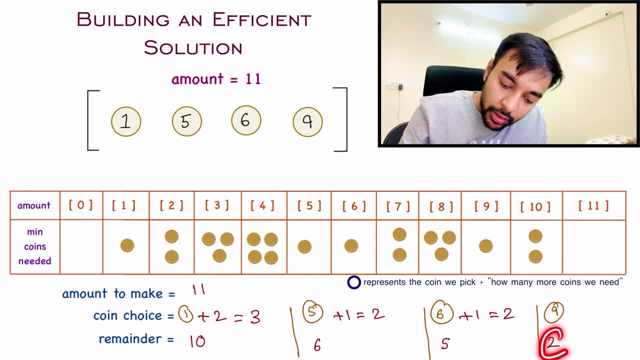 To make a remainder of 5, you need just 1 more coin, And to make a total of 2, you need 2 more coins. Out of all of these 4 values, 2 is the minimum. So to make the amount 11,, you will need a total of 2 coins. 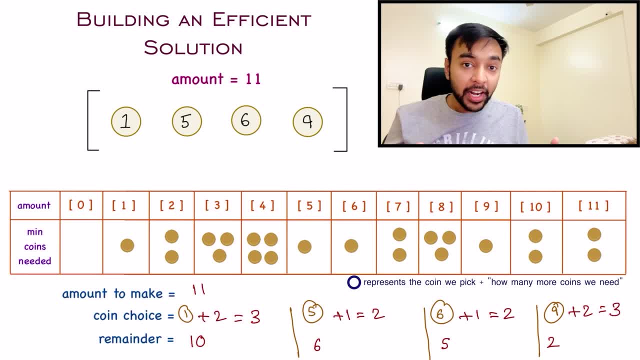 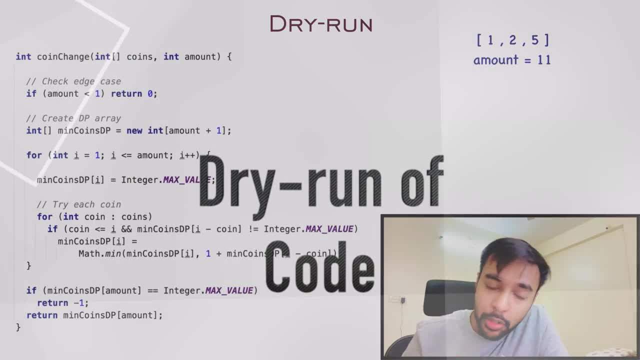 And you can see how we were able to reuse all of our results. Right Now, let us quickly do a dry run of the code and see how this works in action. On the left side of your screen, you have the actual code to implement this solution. 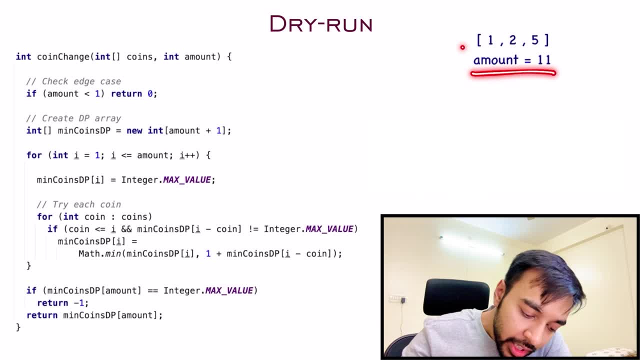 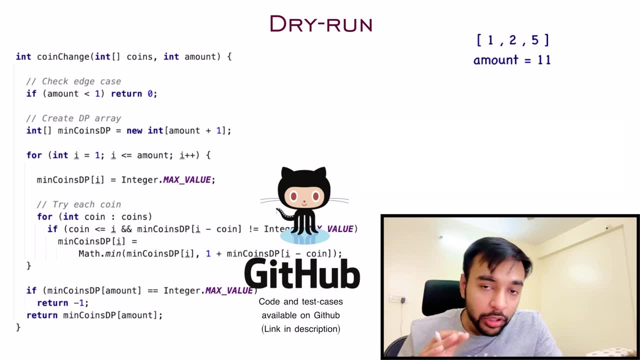 And on the right I have the sample array with me and the amount 11 that are both passed in as an input parameter to the function coin change. Oh and, by the way, this complete code and its test cases are also available on my GitHub profile. 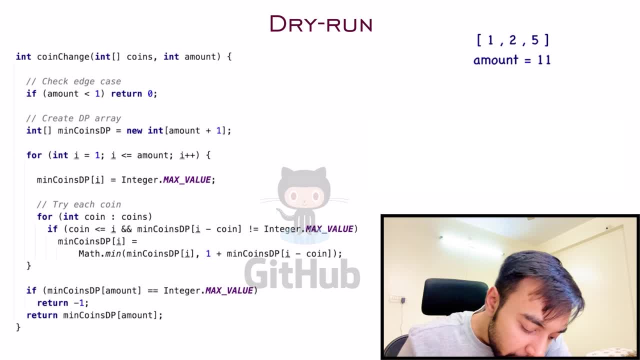 You can find the link in the description below. Moving on with the dry run, we first of all start with checking the edge case. So if the amount is less than 1, we don't have to do anything, We just return a 0. 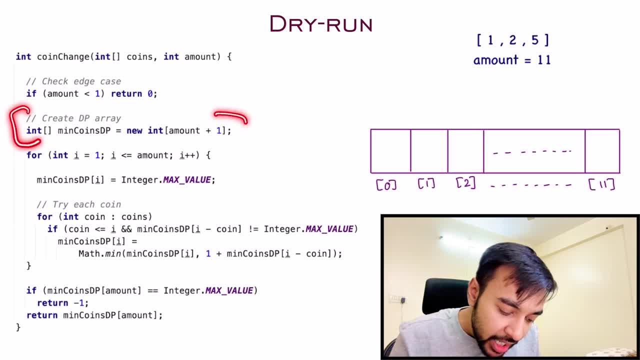 Correct. Now what do we do next? We next create a DP array that will store all of our Memoize results. Right? This array is same as the previous array that we just discussed, Right? So each of these array values will store the minimum number of coins that I need to arrive at that particular amount. 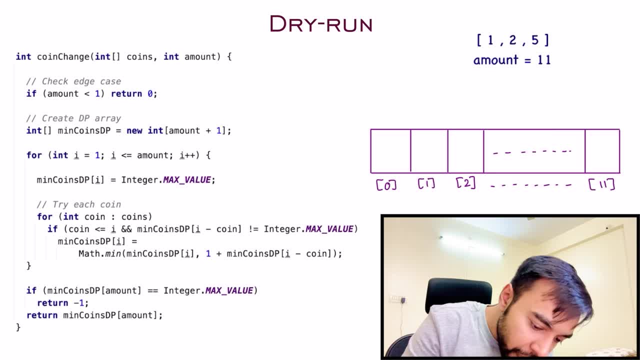 Correct. So now what I'm going to do is I will start a for loop And in this for loop I will start with 1 and go all the way up to the amount Right? So you need to first say okay. To make 1,. how many coins do you need to make 2, how many coins do you need all the way up to to make 11, how many coins do you need And to populate this value? what you will do is you will try each coin. 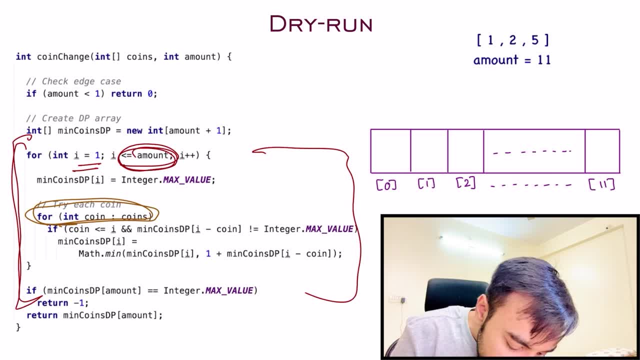 So I start one more for loop, picking each of the coin and then try to determine what is the minimum number of coins that I need to populate each of the value. And that is very, very simple. You will just do a mathmin from the original value that you're picking up. 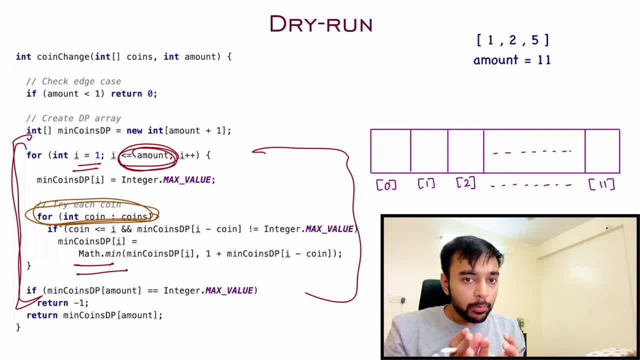 And from one of the value that you're picking in the array. You remember how we picked the minimum value, And this minimum value will now be populated in each of this array element. Once all of this array is filled out, you just need to look at the last value and that is returned as a final output. 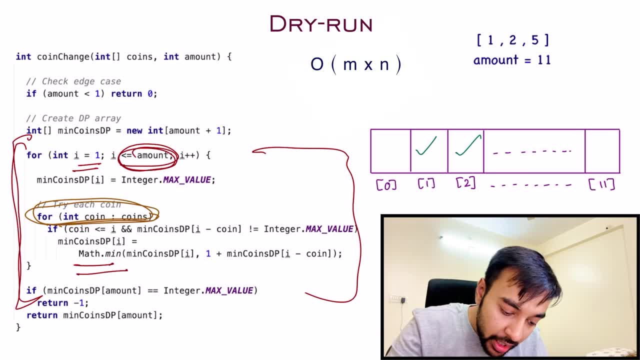 The time complexity of this solution will be order of m cross n, where m is the total number of different coins and n is the total amount that you have to make, And the space complexity of the solution will be order of n, Because That is the array space you need to memoize. 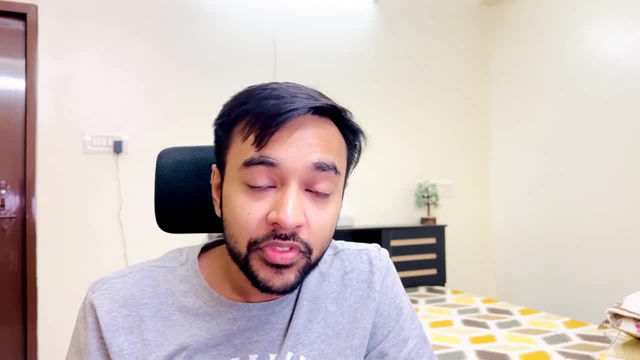 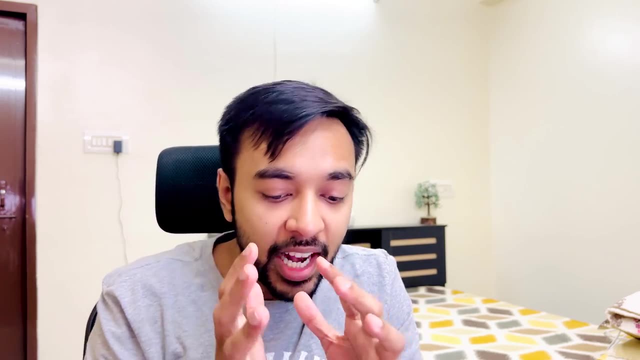 I hope I was able to simplify the problem and its solution for you. As per my final thoughts. I just thought to say that when you solve more and more problems on dynamic programming, you will start to see and visualize some of the patterns, Because problems on dynamic programming have three or four specific patterns. 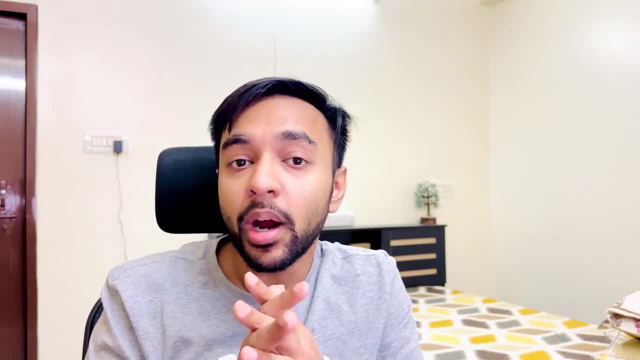 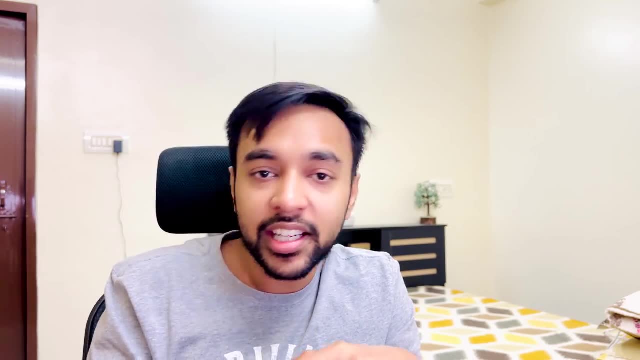 This problem is a variation of the 0-1 knapsack problem, but without any bounds. To understand more about the 0-1 knapsack problem, I have one more video available and you can check the link below. That is much more elaborate and much more visual, with some really good examples.